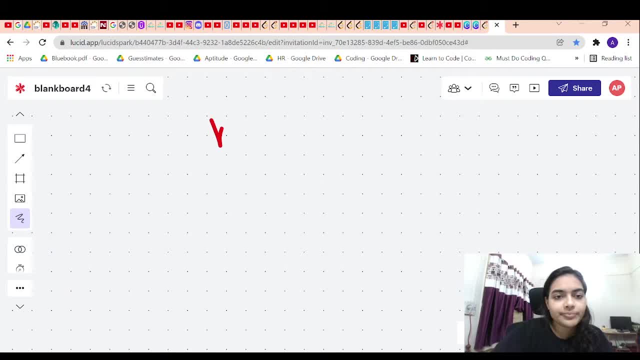 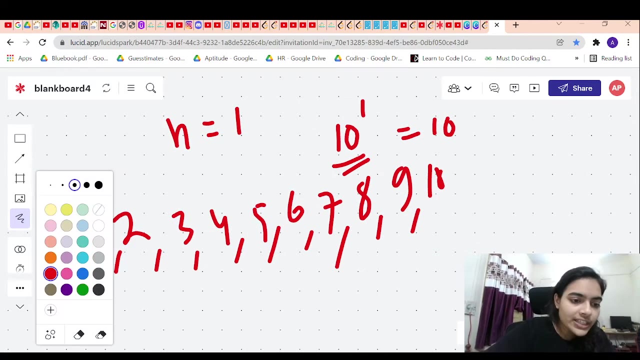 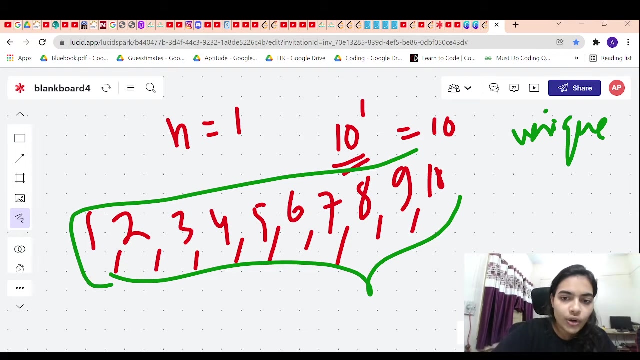 Now let's see the next case For n equal to 1. That means all the numbers up to 10 power 1. This is nothing but 10.. So we have the numbers 1, 2, 3, 4, 5, 6, 7, 8,, 9, 10.. In this, what is the answer? See, all these numbers are the answer, because all these numbers are all consisting of unique digits. 1 to 9 is definitely having all unique digits right, because all single digits are different. 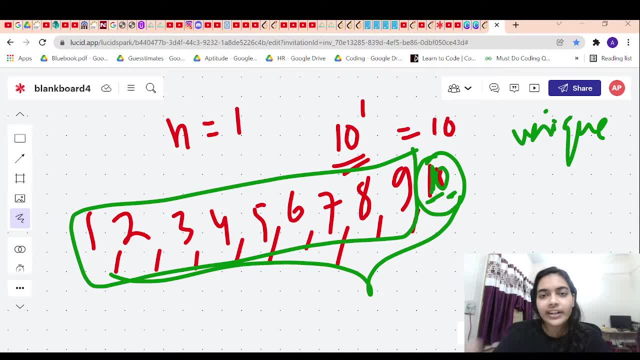 Even the number 10 is having unique digits because 1 and 0 are different. They are unique digits. 1 is not repeating or 0 is not repeating. Both are unique or different digits, right? So in this case all numbers are the answer. So for n: equal. 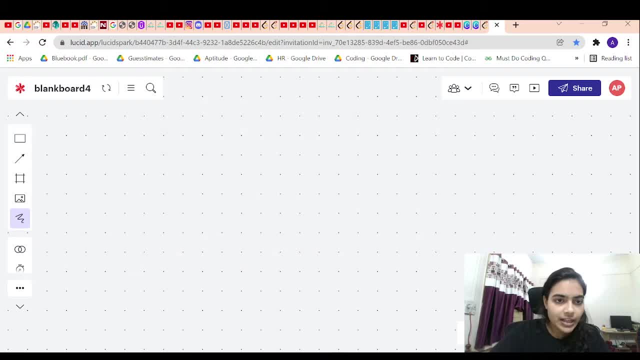 to 1,. the answer is 10, okay, Now let's try to take some other example. What about? okay for n equal to 2?? Now let's try to understand. So for n equal to 2 means all the numbers up to 10 power. 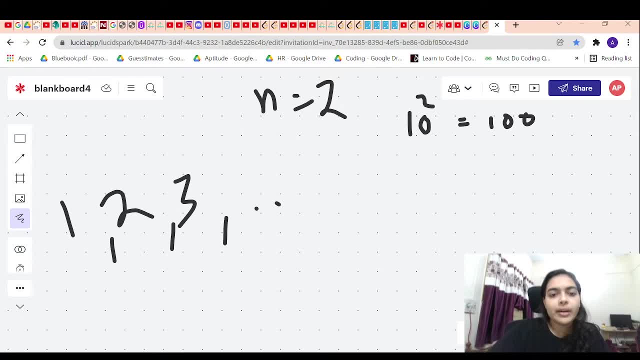 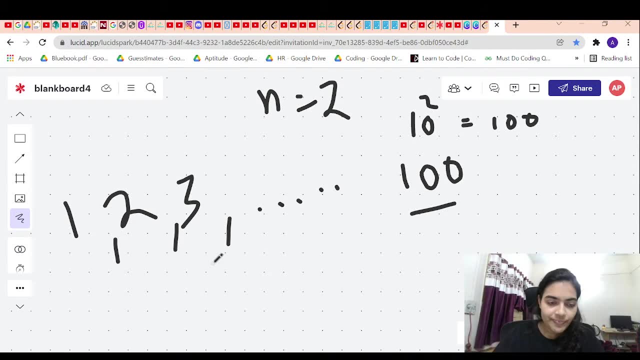 2, which is 100.. So all the numbers 1,, 2,, 3 up to 100, okay, You have to find out how many of the numbers are having unique digits, okay, So, for example, if you have number like 63, okay, which? 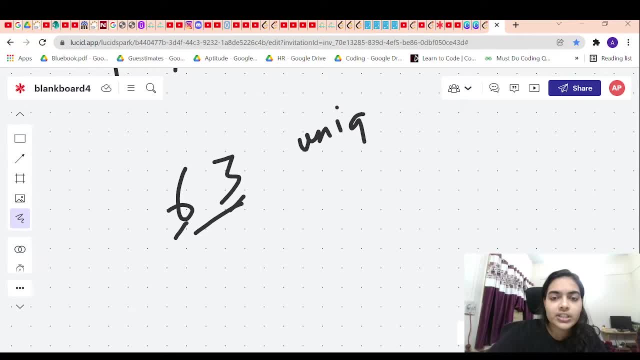 is lying in this range. it is having both digits unique, right, Because none of the digits are repeating. So this is a unique number, okay, But what about 66?? This is not having unique digits, right, So this should not be included in the answer 78,. 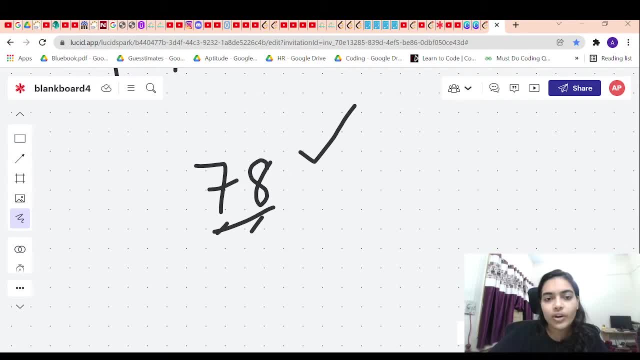 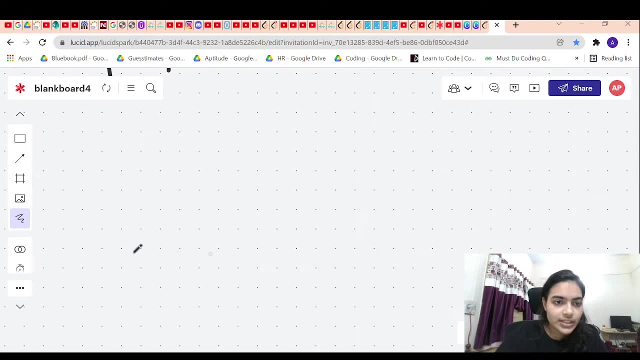 is having unique digits, right. Neither 7 or 8 is repeating, But 88 is not having unique digits. 77 is not having unique digits. okay, How do we build the answer for this? See, the simple approach is: okay, let's. we have already seen single digit numbers. We definitely know all the 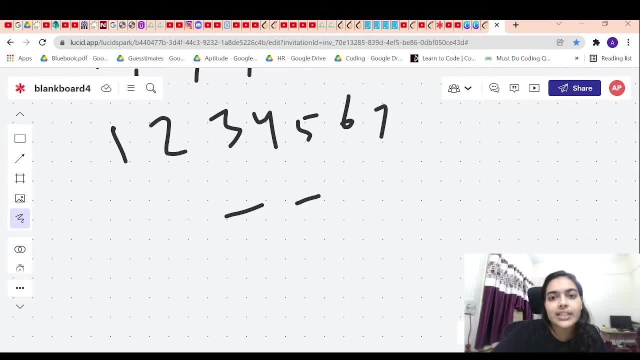 single digit numbers are going to be unique, okay: 1, 2,, 3,, 4,, 5,, 6,, 7,, 8, 9.. All these numbers are definitely going to have unique digits. So we at least have 9 numbers, okay. Now what about the? 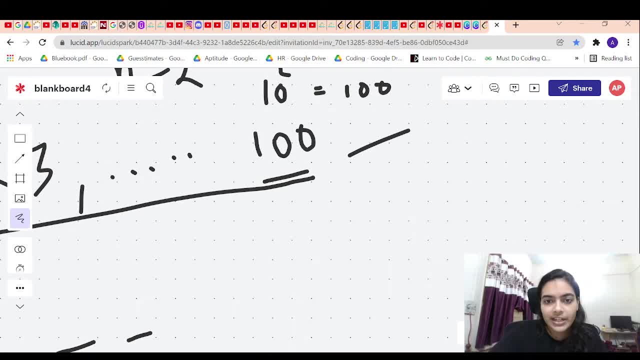 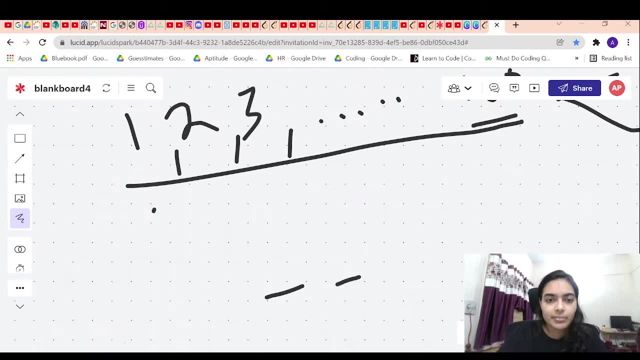 double digit numbers. okay, 1 to 100 consists of two types of numbers. 1 to 100 consists of numbers, right? So 1 is single digit numbers. All single digit numbers are unique. What about the double digit numbers? How do we take care of the double digit numbers? So see when we are. 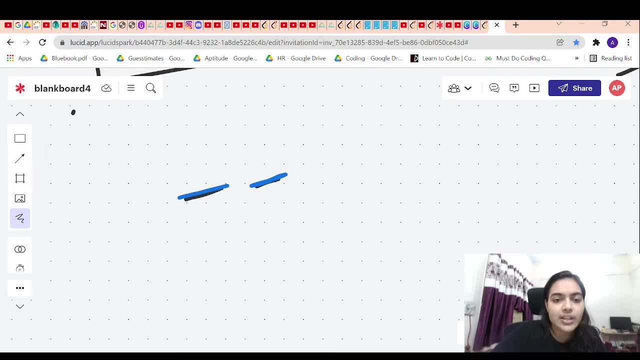 looking at the double digit numbers, it has two digits right. One is the 1's place and one is the 10's place. okay, Now see- let's think of the 10's place- What all values can come here. 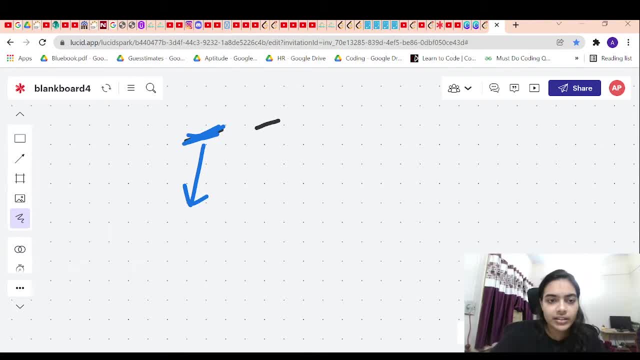 Can you have 0?? You cannot have 0, okay, Because first digit, if it is 0, it will be just a single digit number, right? So you cannot have any other values. So 1,, 2,, 3,, 4,, 5,, 6,, 7,, 8,, 9.. You can fill. 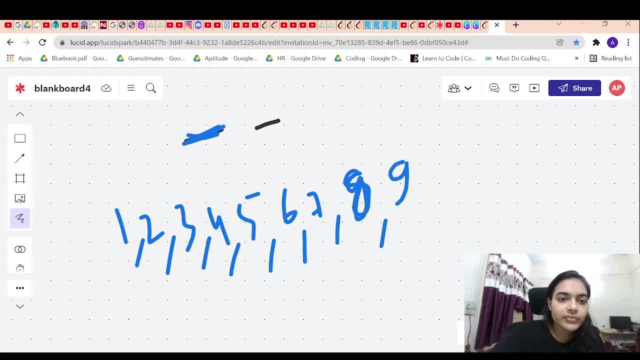 any value- right, You can fill any value here. Let's say you fill 8, okay, Randomly. let's say I fill 8, okay, Without loss of generality. let's say I am filling any value- 8, okay- Among the 9. 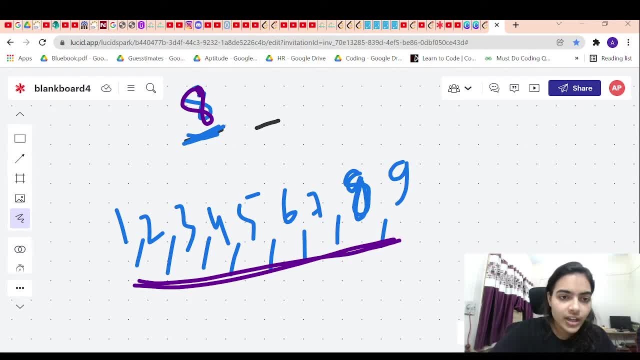 choices that I have. I had 9 choices. I am filling 1 choice. okay, In the first digit. Now what about the second digit? Now, second digit cannot take the value 8.. So your choices reduce to only 8 choices. 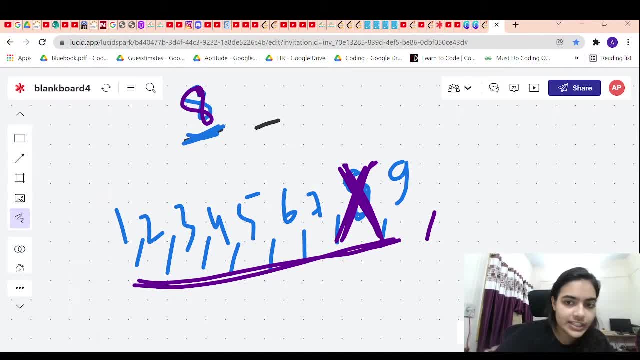 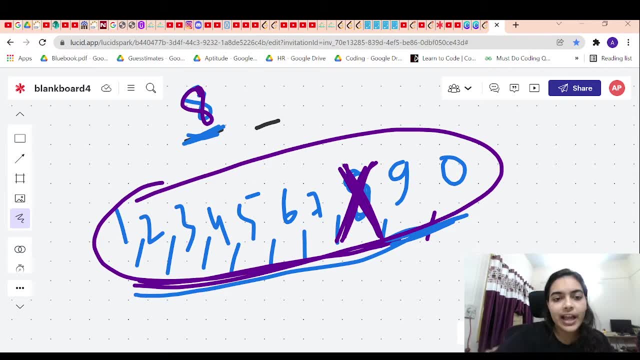 but second digit can also be 0, okay, Second digit can also be 0, okay. So again, you have 9 choices. okay, Second digit can be 0.. You can pick any of the numbers and you will not have a. 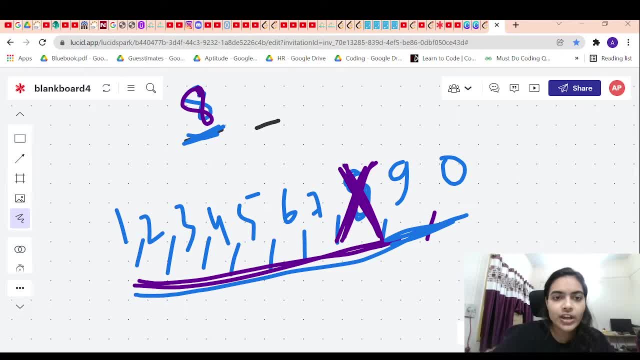 repeating digit. Except 8, you can pick any of these 9 numbers, okay. So again you have 9 numbers. Let's say, without loss of generality, you pick 85,. okay, So this is how you form a 2-digit number. 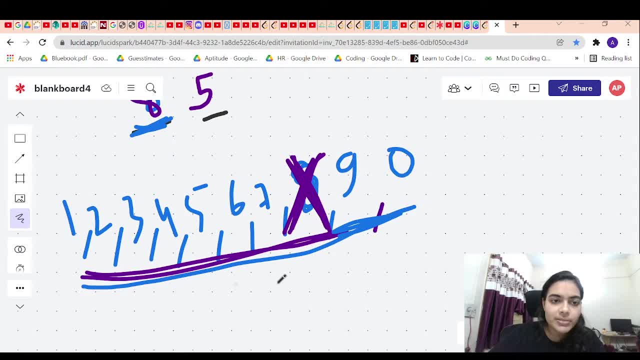 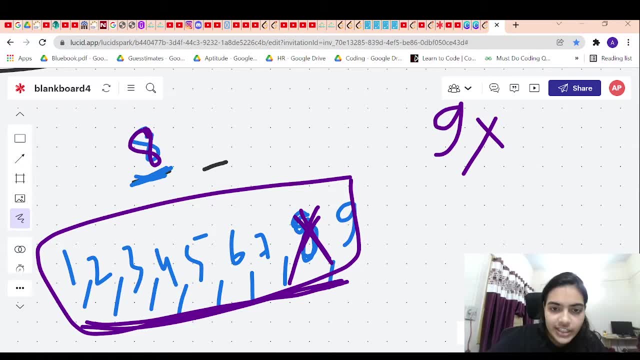 which is not having any repeating digits. So how many possibilities were there? For the first digit, you had 9 possibilities right For the first digit, And for the second digit 1 digit got removed but 0 also got added, So again you have 9. 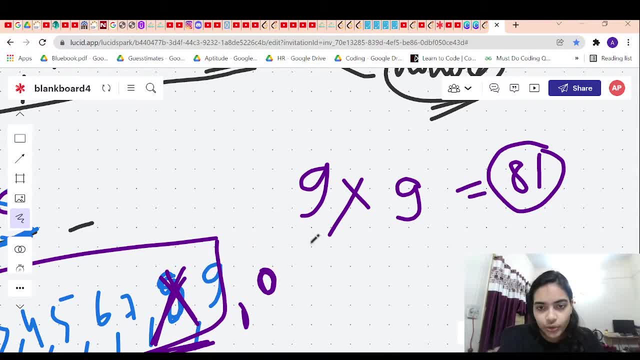 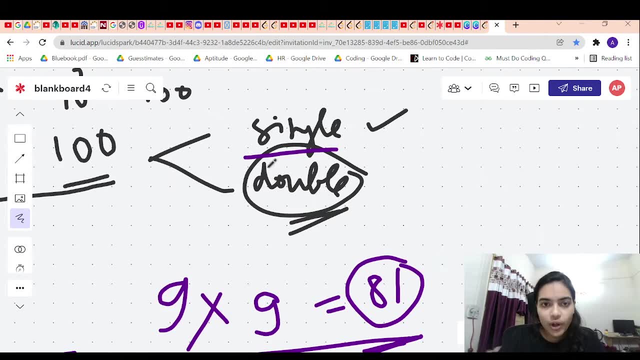 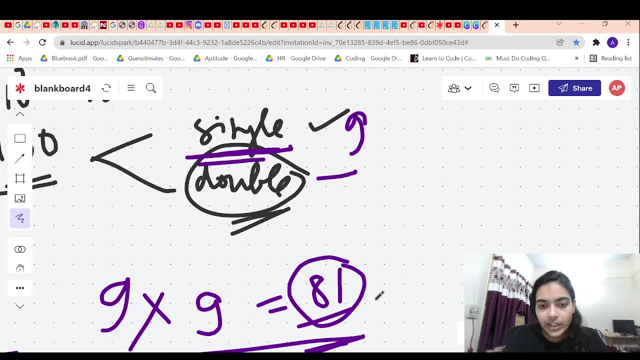 possibilities. So you have 81 choices. okay, So you have 81 choices, okay. And what about the single digit numbers? right, So you also have the single digit numbers. So, since you have the single digit numbers, you have 9 choices here. okay, 81 plus 9, okay, 81 plus 9 is 90.. And if 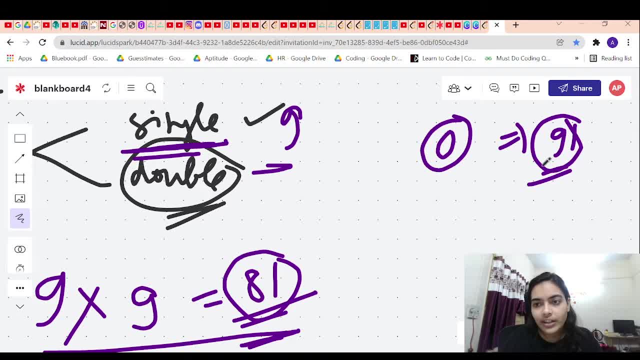 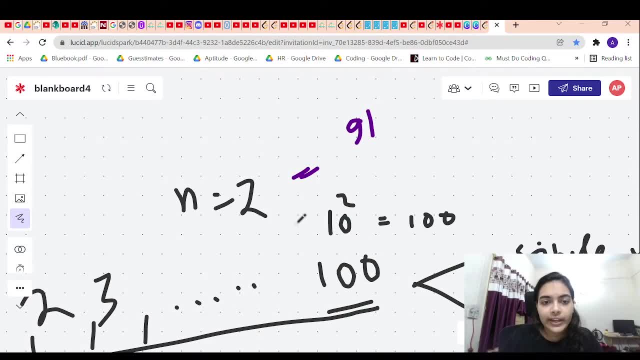 you have 91 choices. okay, So you have 91 choices. So the answer for n equal to 2 is what It is: equal to 91,. okay, Now let's quickly build the answer for some other. okay, n, Let's say we have. 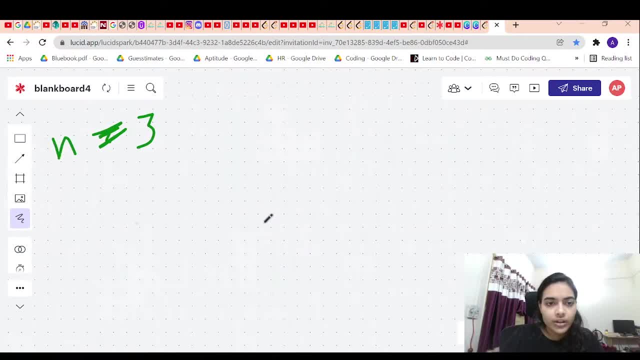 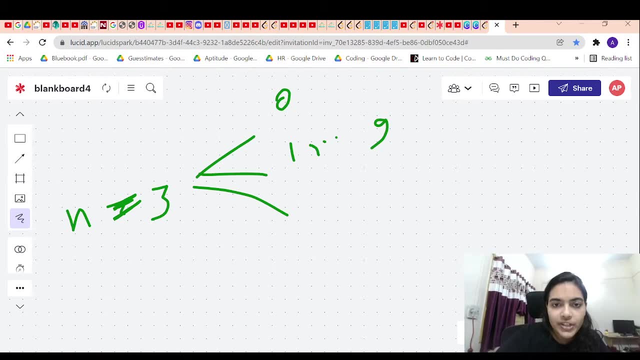 n equal to 3.. Let's quickly see the answer now. So see, for n equal to 3, what are we going to do? See, 1 number is 0.. 1, we have numbers from 1 to 9, right, 1,, 2,, 3,, 4,, 5,, 6,, 7,, 8,, 9.. Single digit: 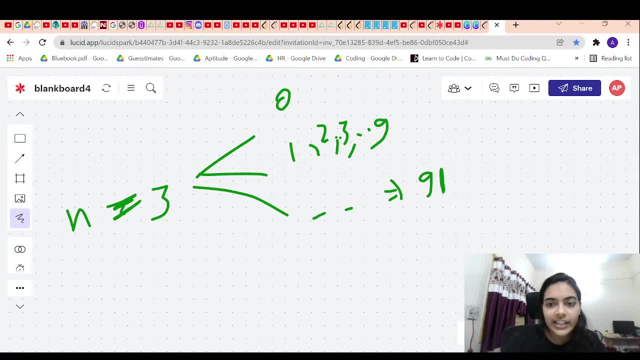 numbers And then for double digit numbers. we already know we have 91 numbers. okay, We have 91 numbers. Now let's see for n equal to 3, how we will solve the problem. So for n equal to 3,, 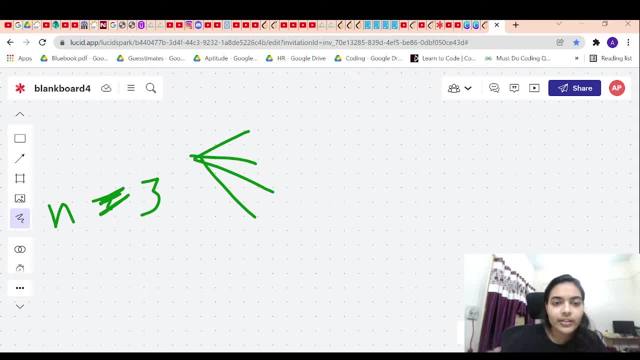 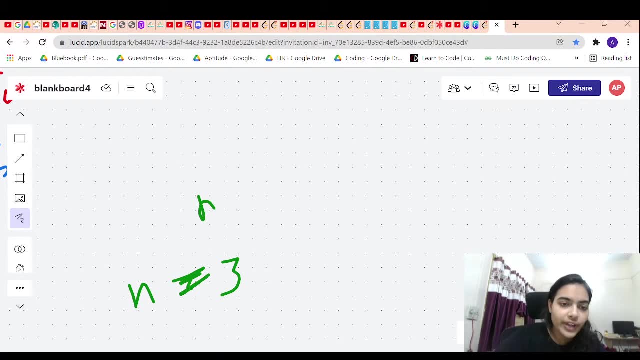 what will be the answer. See, you already have okay for n equal to 3,. you already have the answer For n equal to 2, we have already seen. For n equal to 1, we have already seen. 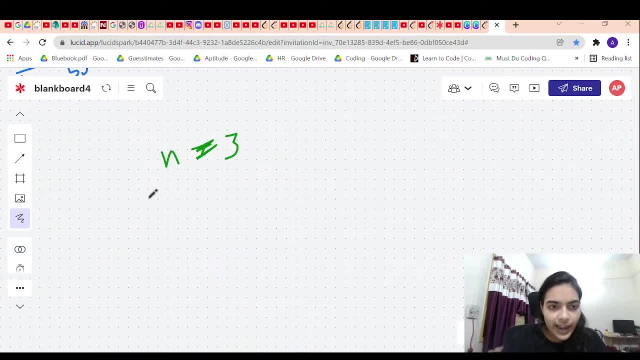 For n equal to 0, we have already seen. Now let's try to see the answer for n equal to 3.. Let's see for single digit numbers first of all. n equal to 3 means okay, first of all. 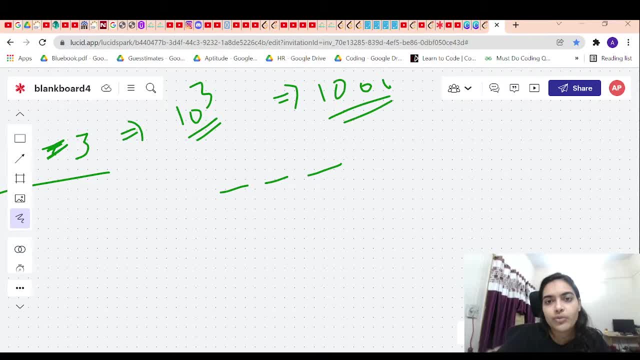 up till 10 power 3. That means all the numbers that are less than equal to 1000.. So that will be okay. that will be single digit numbers And 1000 will never be the answer. 1000 cannot be answer. 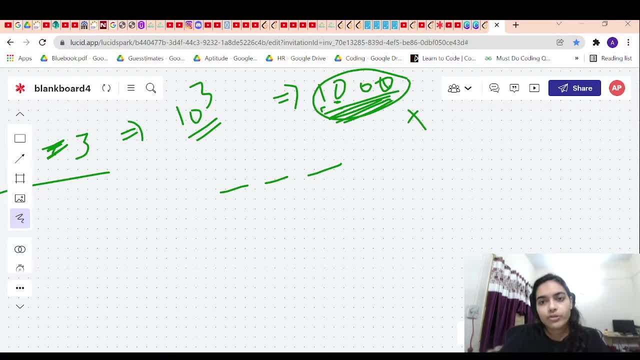 because, see, in this case 0 is repeating right, So 1000 will not be the answer, So you just need to take care of numbers less than 1000.. So we have already seen how to find for double digit numbers. 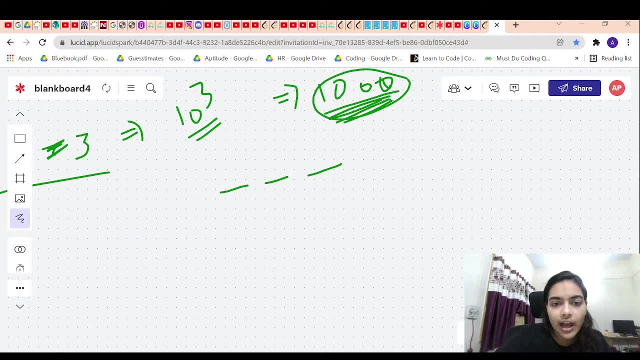 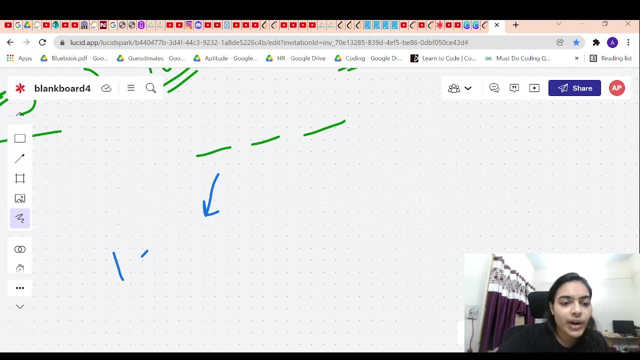 We have already seen how to find for single digit numbers and all. So let's see how how to find for triple digit numbers. So for triple digit numbers, first digit can take how many combinations: 1, 2,, 3,, 4,, 5,, 6,, 7,, 8,, 9.. Any of the 9 choices You can. you have 9 choices for. 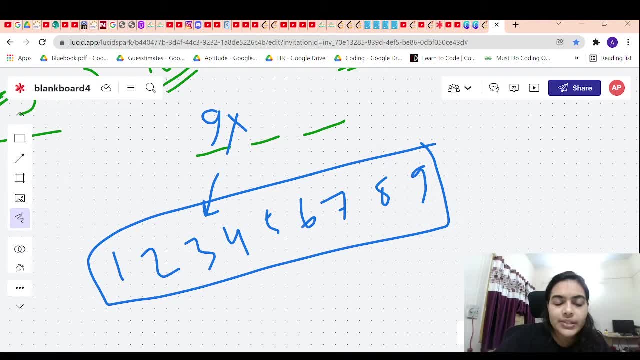 the first digit. What about the second digit? Second digit: one of the digits will get removed, right? Whichever digit you pick, without loss of generality. let's say you pick this, So you have only 8 choices, but 0 also gets added, So again you have 9 choices. okay, Now for the third digit. 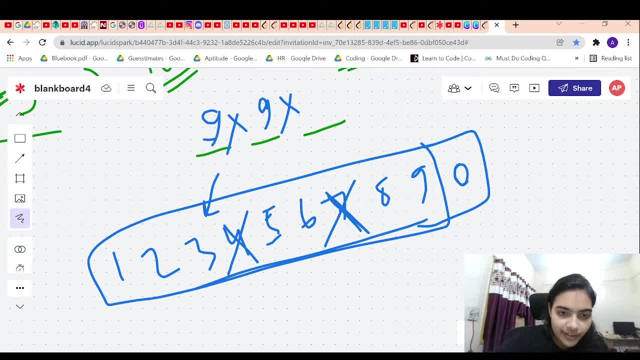 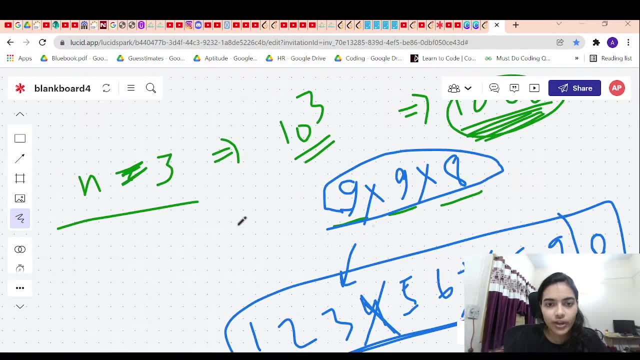 okay. Without loss of generality, let's say we pick this digit okay. So now you have 8 choices. So for a 3 digit number, you have 9 x 9 x 8 choices. okay, And for a 2 digit number, you had 9 x 9 choices For a single. 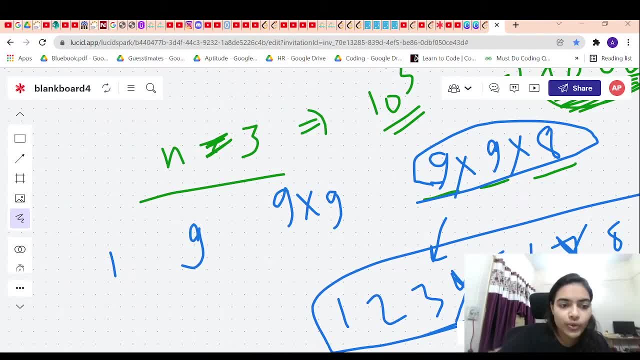 digit number. you had 9 choices. okay, And simply, if you take 0, you have 1 choice, So you should add all these answers. If you add all these answers, you will get the answer for n equal to 3,. 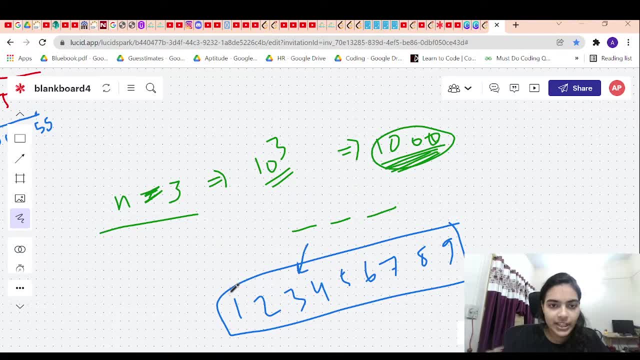 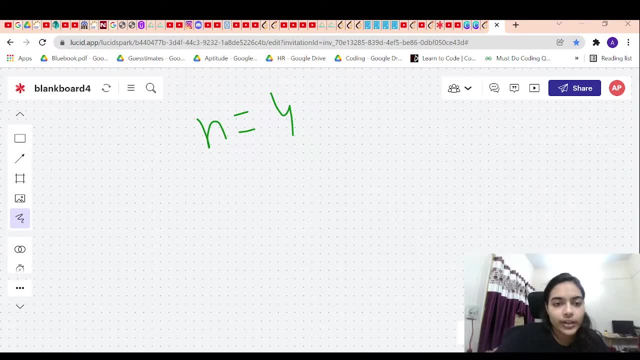 okay, So this is the simple logic. Now let us quickly see for some other case. Let's see for n equal to 4, and then we'll move forward to coding it. okay, So for n equal to 4, what is the answer? So for the first digit, you have 9 choices, right? 1,? 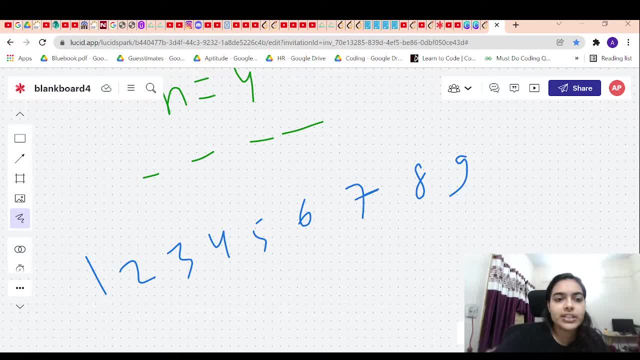 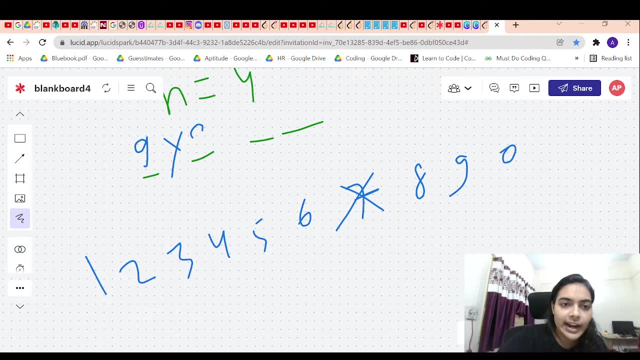 2,, 3,, 4,, 5,, 6,, 7,, 8, 9.. For the first digit, you have 9 choices, okay. For the second digit, okay, One of the choices will get removed but 0 will get added. So again you have 9 choices. 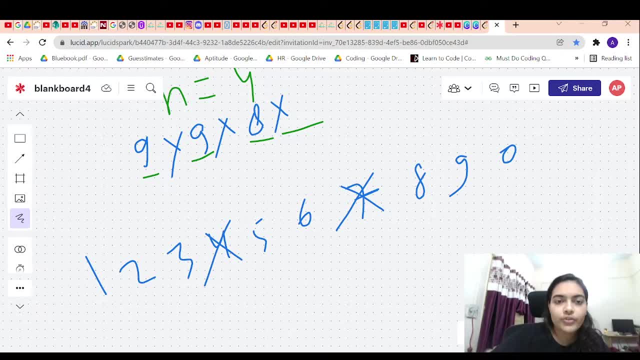 For the third digit, one of the choices will get removed. So you have 8 choices. For the fourth digit, one of the choices will get removed. So you have 7 choices. For 4 digit numbers. these are the number of ways you can make a choice. So for n equal to 4,, you have 9 choices, So you 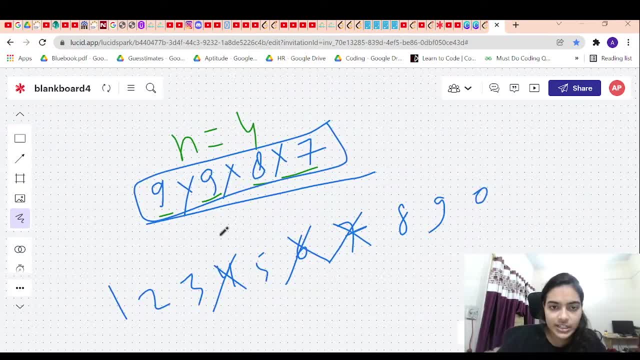 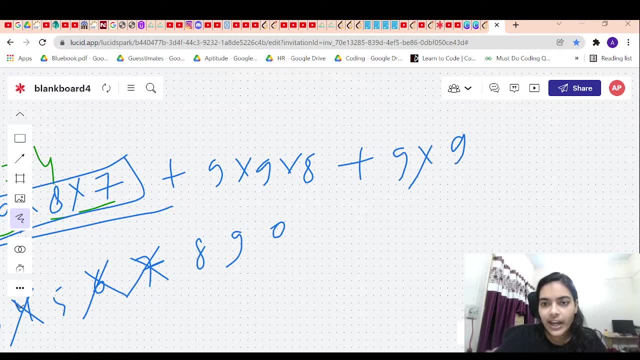 4 digit numbers with unique characters. okay, Unique digits. For a 3 digit number, what was it? It was 9 into 9 into 8.. For a 2 digit number, it was 9 into 9.. For a single digit, it was 9.. And 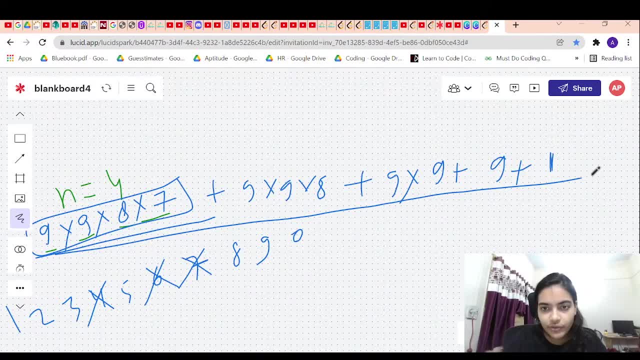 for simply 0, you have 1.. So if you add all these values, right, If you add all these values, then in that case you will get the answer for n equal to 4.. Now coding this is simple, right Once. 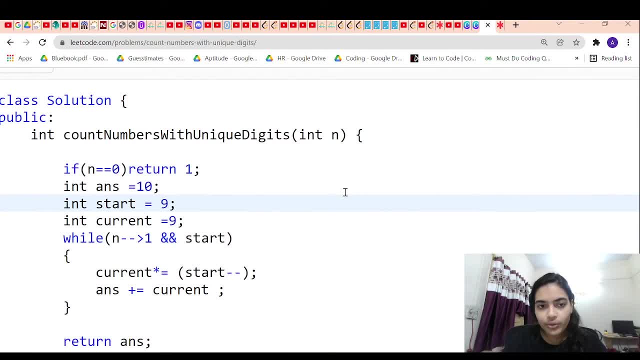 we know the approach. coding this is simple, So let's move forward to coding it. If n is equal to 0, you can return 1, okay, Otherwise you can return 1.. So you can return 1.. So you can return. 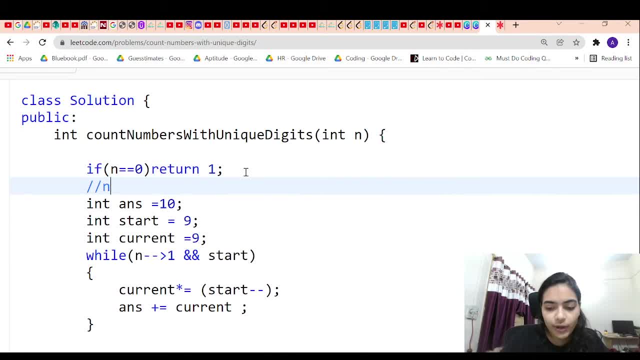 2, right. So for n equal to 2, right For n equal to 1 and forward, let's see: For n equal to 1, the answer is simply 10, right For n equal to 1, we have the answer directly. Answer is 10 because 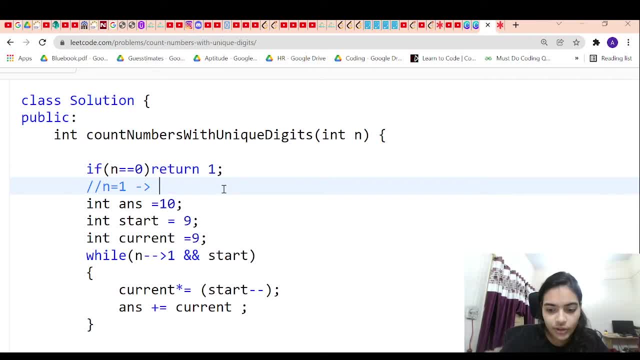 you have 9 single digit numbers, okay, And you have a 0,. okay And you have a 0. So that is why you have total 10 numbers, all the single digit numbers, and 0.. So for n equal to 1,, the answer is: 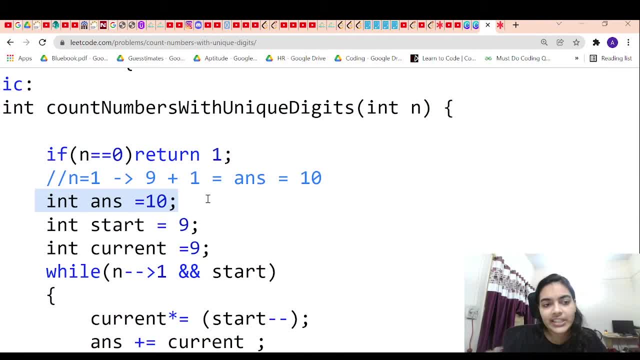 simply equal to 10, okay, So that is why you have a total of 10.. So you can return 1, and you can. we are starting from the base case. we are starting from n equal to 1, so the answer is 1, okay. so if 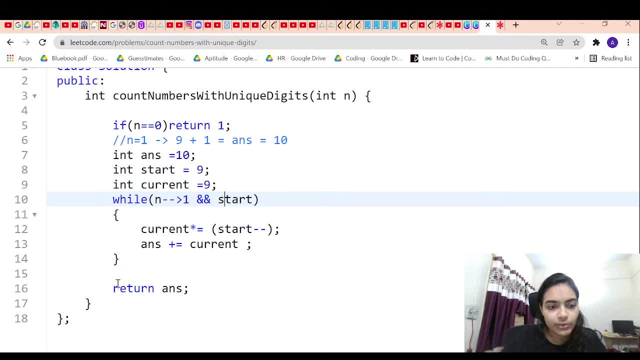 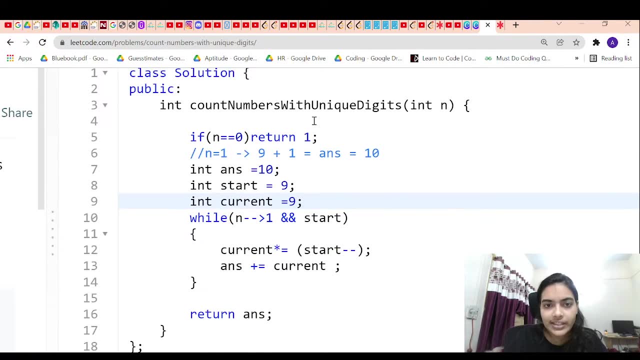 if n is equal to 1, it will not even run in this while loop, and you will. you can. you can simply return 10, okay. but for all other cases, okay, let's say let's do a dry run of this code, okay, let's try to find out the answer. for, let's say n equal to 3, okay, we'll do a dry run for uh, starting uh. 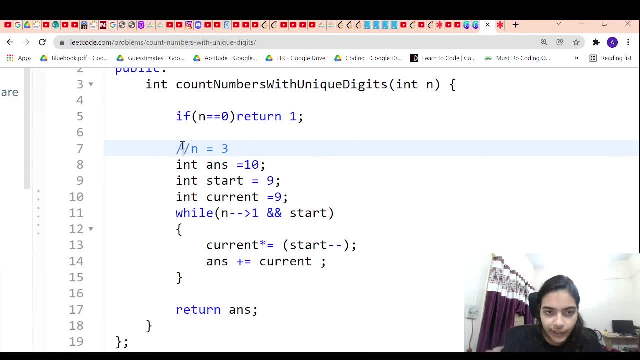 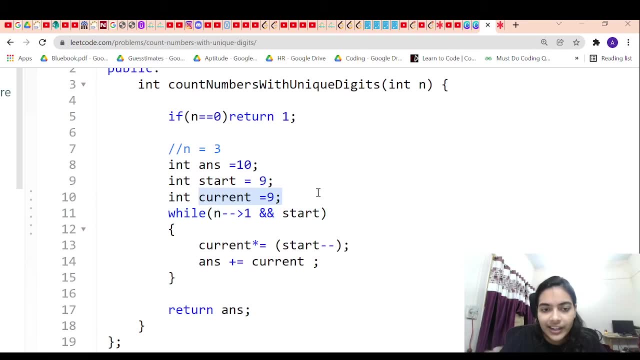 from n equal to 1, 2, 3. so we'll go up to n equal to 3 and we will see the answer, whether we are getting the correct answer or not. okay, so we are starting with the first digit, which is 9, and the current digit, which will keep on changing, right. for example, see here: you have nine choices. 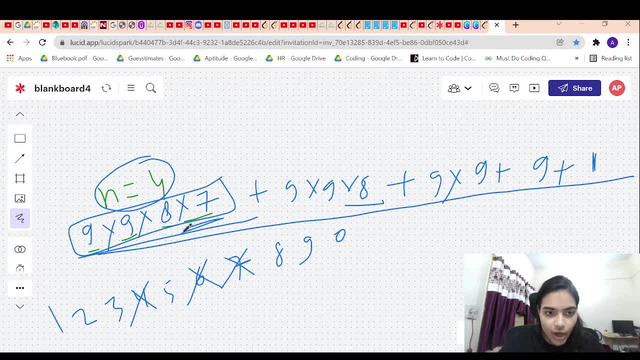 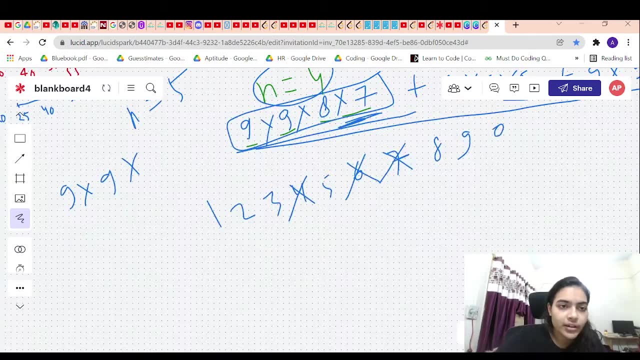 then your choices keep decreasing right. next time you have eight choices, next time you have only seven choices. okay, if you had n equal to five also, then in that case what would have happened? you would have to consider the five um five digits also. so then it will become: 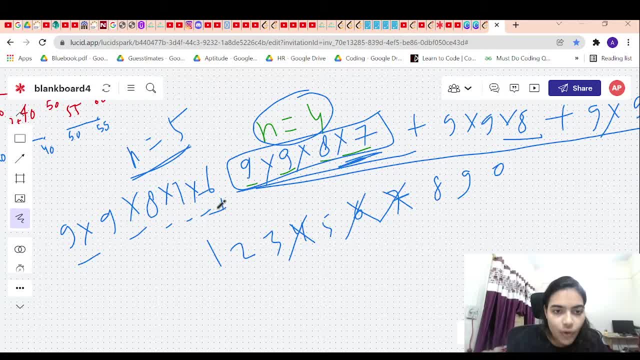 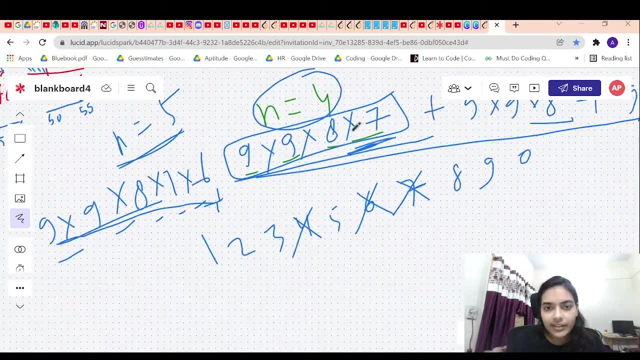 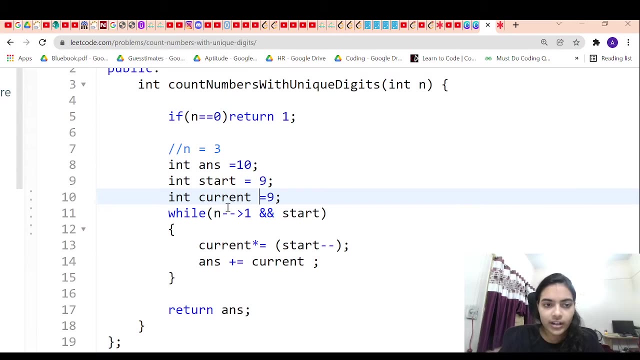 6, it will become 9 into 9, into 8, into 7, into 6, right, so you will have all these choices also. so there is a variable current, which is representing this variable that is decreasing: first nine, then eight, then seven, then six, the digits as the digits keep on increasing your 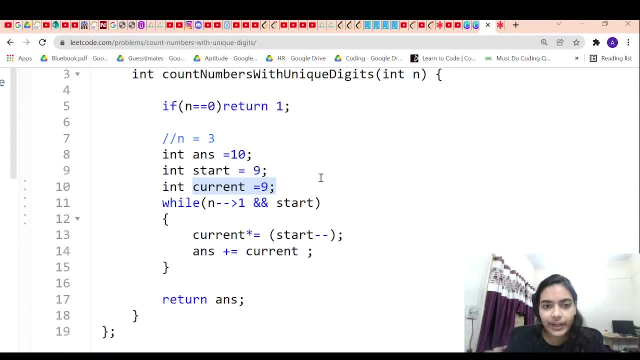 number of choices, number of options for the digits keep on decreasing, right, so that's the current variable. initially we are starting from nine and then we keep, uh, decreasing. so that's what i am doing. okay, let's do a dry run of this. so for um start, initially, our n is equal to 3, right, let's let's find the answer for n equal to 3. 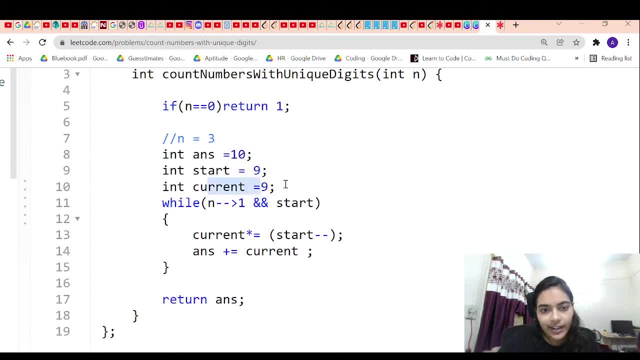 so your answer is 10. start is 9. current is 9. okay, now we will enter into the while loop. okay, n minus minus is greater than 1. okay, and start is also equal to 9. so both the conditions are satisfied. now what will happen to the current, your current, okay, current is starting with 9. 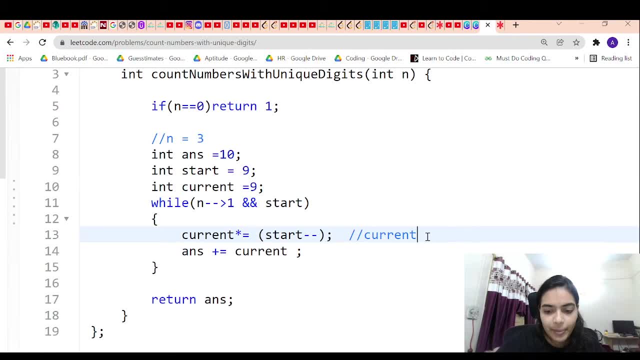 okay, because you have 9 options for a single digit number. now what will happen to current? current will become equal to 9 into what start minus minus. so first it will multiply, then this minus minus will apply. so first it will become 9 into 9. okay, so current will become equal to 81. 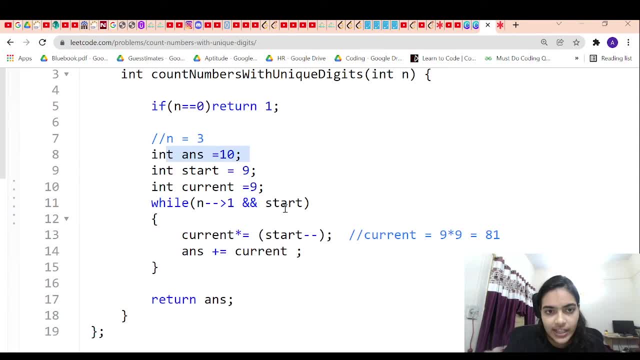 in this case, and your answer will get added. what is your answer? answer is already 10. right, answer is already 10, because why is it already 10? for n equal to 1, the answer is 10. okay, now in this case. so let me break it up and write for 0. okay, the answer is 1. okay, simply. 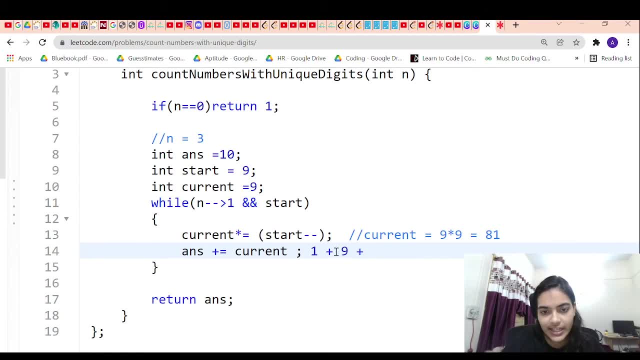 1 and then for a single digit numbers, you have the answer is 9. okay, so basically, for n equal to 1, the answer is 10, 1 plus 9, which is 10. and also now what will happen? current will get added to answer. 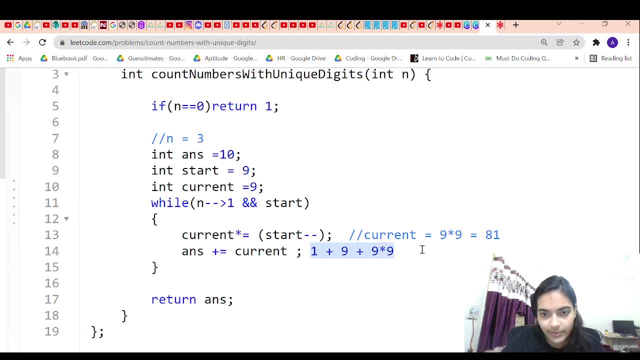 so 9 into 9 will get added to the answer, so your answer will become equal to this entire value. this is 10 plus 81, this is 91. so right now your answer is 91. okay, now let us go in the next iteration of. 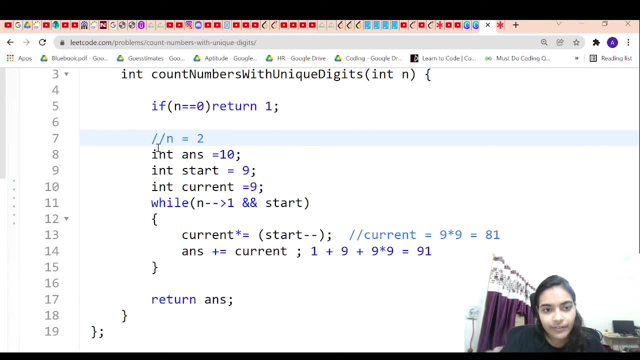 the while loop. so now, n will decrement, right, n will decrement, n will become equal to 2 to. because of this case, n will decrement. it is still greater than 1 right, so this is still valid. so in this case, let us go to the next condition. so what will your current will become. current will become. 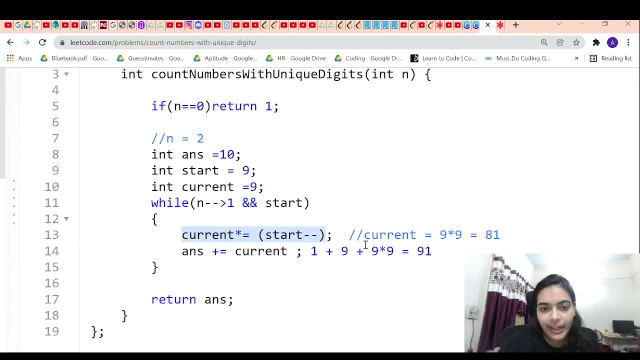 equal to current will again multiply, start will decrement and current will again multiply with the next value. so start would have become equal to 8, right? so this time current will be equal to 81 into 8. so what will current be? current will be 8. ones are in the 64 648, right. 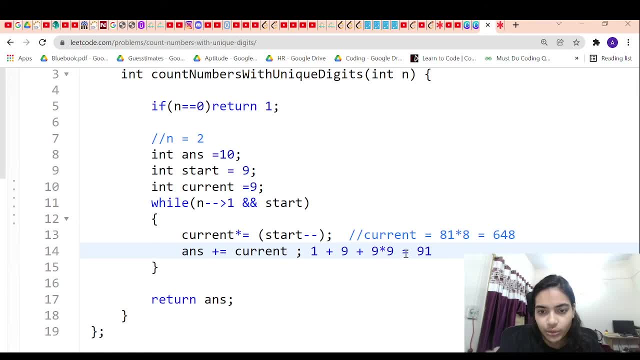 so current is equal to 648, so answer will get added to. so 648 will get added to answers. what is 648? 648 is equal to 9 into 9, into 8, that's it. so this will also get added to the answer. whatever is this value, 648 plus 91, what is that? 8 plus 1 is 9, 9 plus 4 is 13, and then you have. 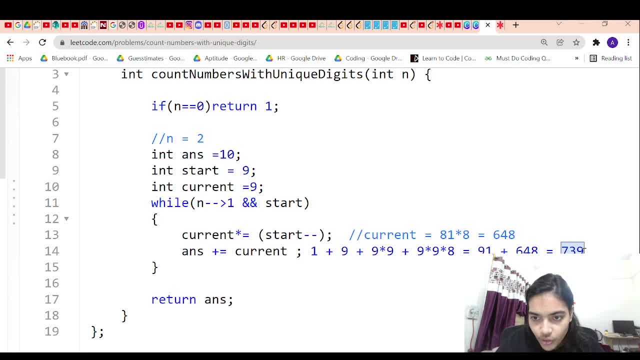 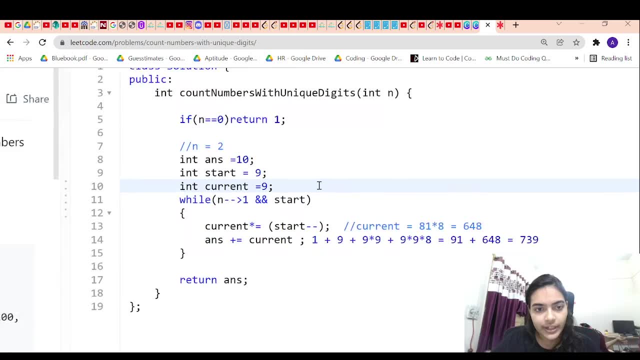 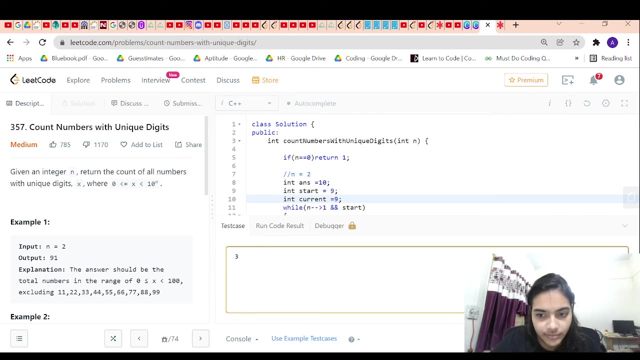 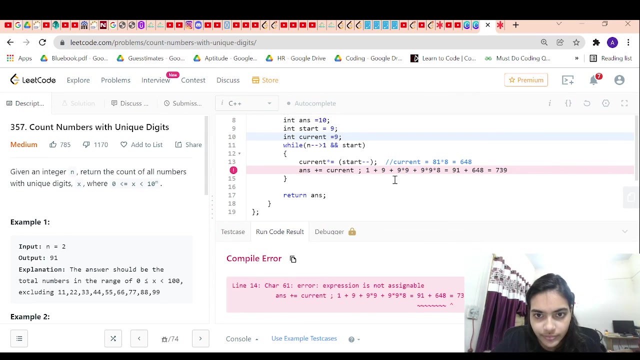 6 plus 1 is 7, so it should be 739, right, and then you can return the answer. so next time when you enter into this loop, it should exit. so let us do a test case for n equal to 3. let's see if it is working. okay, i should give.